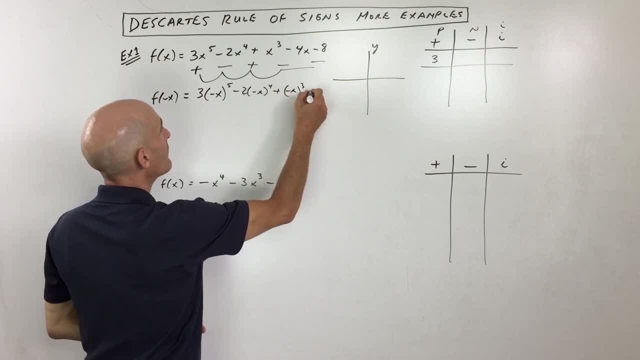 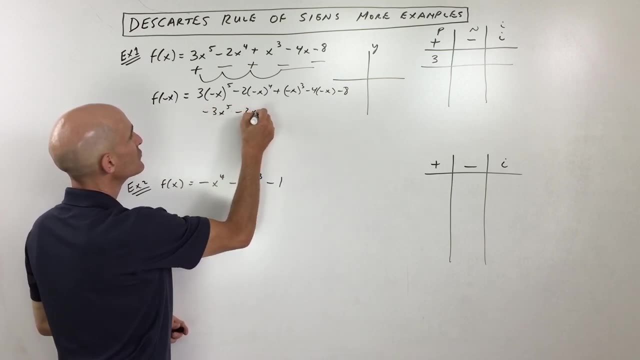 4th, plus negative x cubed minus 4 times negative x minus 8.. If we go back and simplify, we get negative 3x to the 5th, negative 2x to the 4th, negative x cubed, positive 4x to 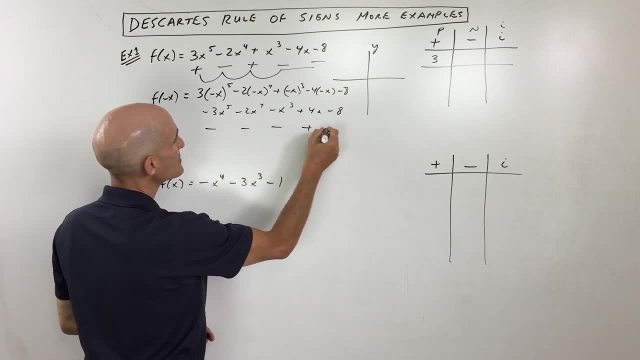 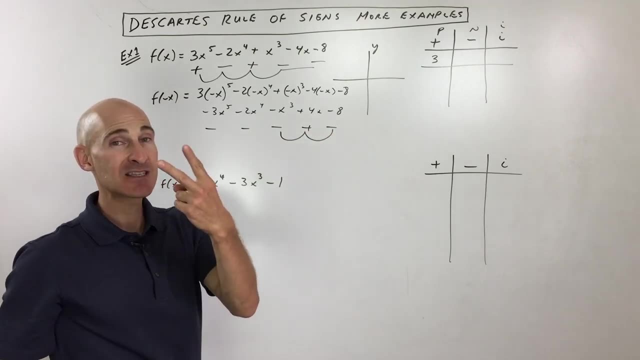 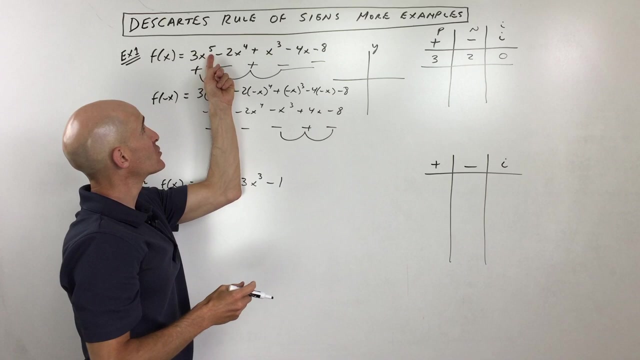 the 4th and negative 8. So we've got a negative, negative, negative, positive negative. So here you can see it's changing once twice. So what that tells us is that we have a maximum of two negatives. And then if we add across here, 3 plus 2 plus 0 equals 5, it should. 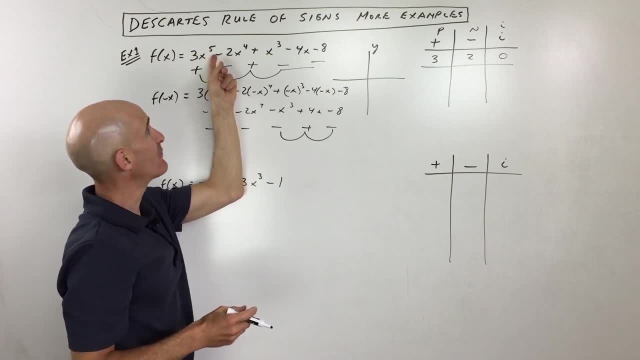 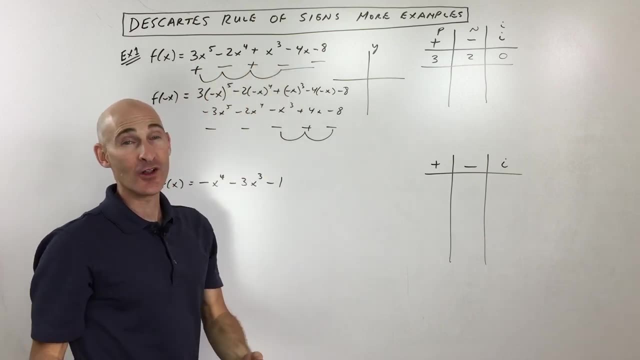 always add up to this highest degree of the polynomial- okay, 5 in this case. Now the other thing that's interesting is that if the coefficients of your polynomial are all right, then what happens is if your zeros come, if you have any imaginary zeros, they 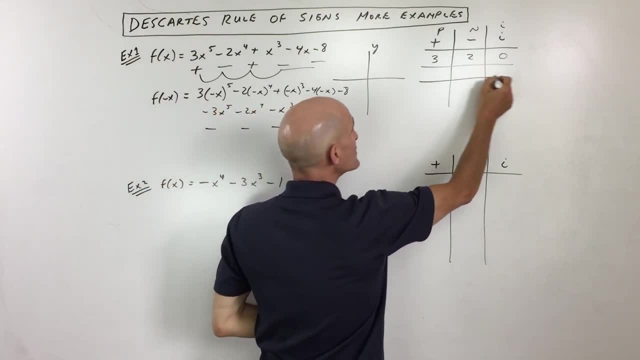 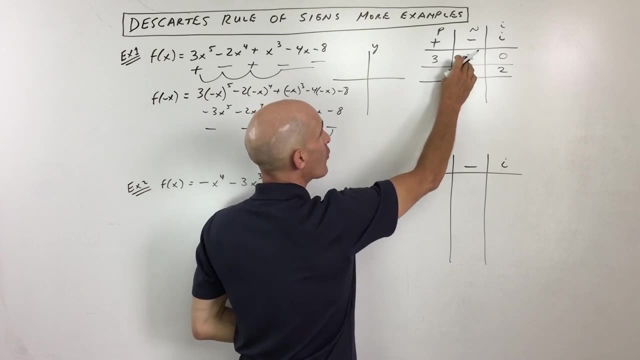 come as conjugate pairs. So what that means is, for example, if we had two imaginary zeros, then what happens is we have to decrease the number of positive zeros by 2 or the number of negative zeros by 2.. So we always go down by 2,, 4,, 6,, 8, by an even number, right, an? 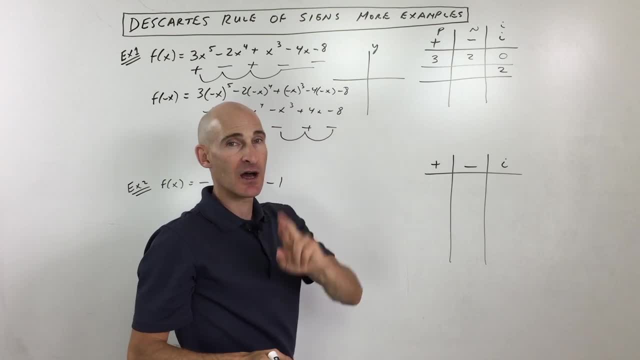 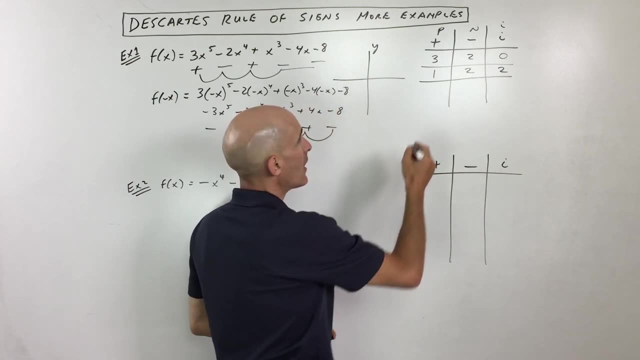 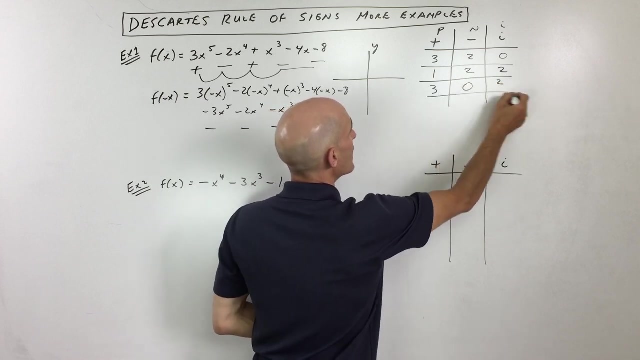 even amount because of these imaginary ones coming in conjugate pairs. So in this case, another possibility is we could have one positive, Two negative and two imaginary. Another possibility would be we could have 3 positive, 0 negative and 2 imaginary. Another possibility: we could have 1 positive, 0 negative and 4 imaginary. 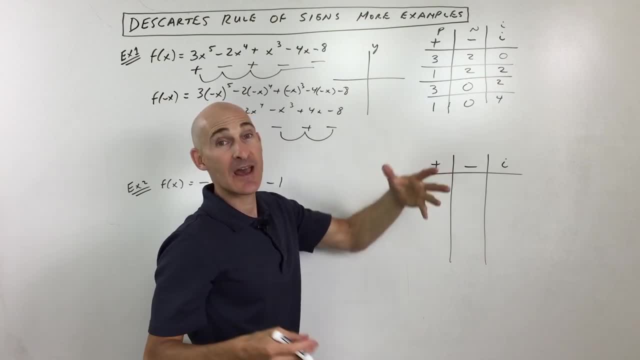 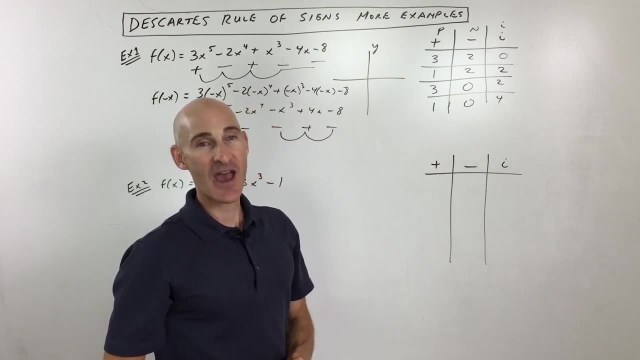 Now, I can't take another 2 away from this 1 and make this a negative 1.. You can't have a negative number of zeros, So these are our only combinations here. Now you're probably asking yourself: well, Mario, why does this even matter, right? Well, here's the thing. 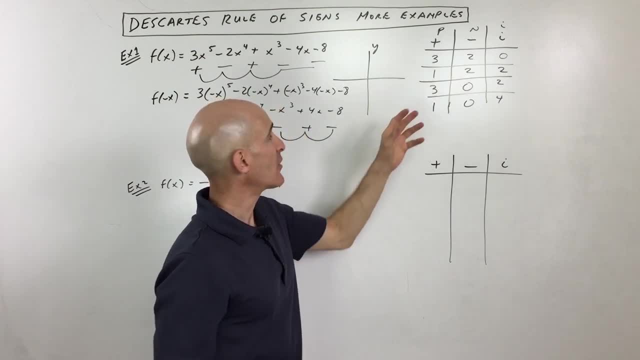 If you're trying to use your rational zero-threatening formula, you're going to have to use your rational zero-threatening formula. If you're trying to use your rational zero-threatening formula, you're going to have to use your rational zero-threatening formula to calculate the. 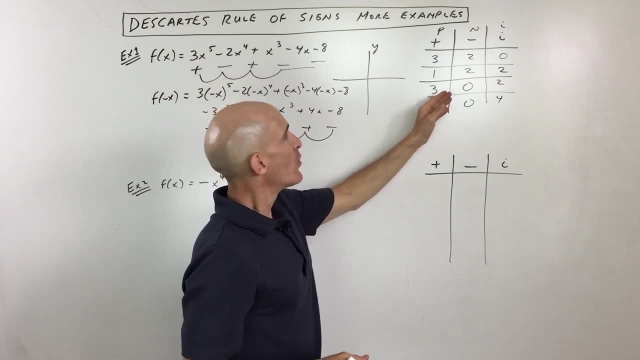 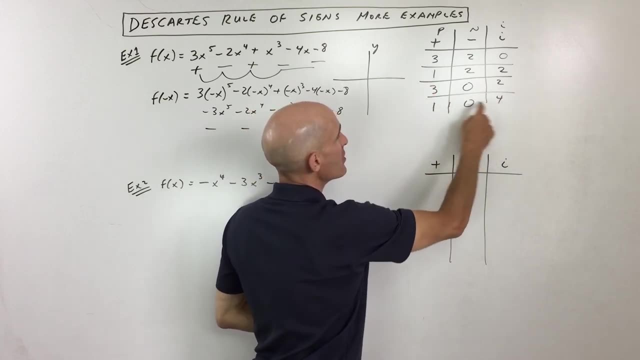 zeros, the P over Q method you probably learned in your class. What you can do is you can be strategic. You can say: well, I know that there's at least one positive zero. If it's this scenario, here or here there might be no negative zeros. So what you can do is you.